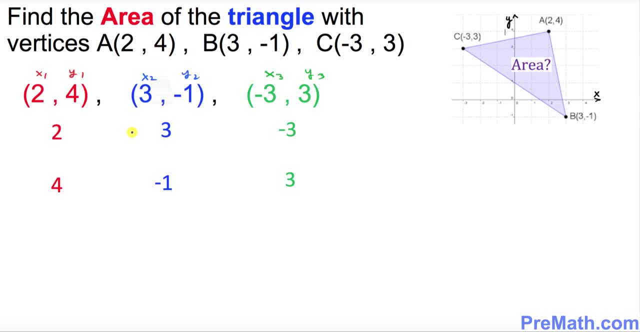 and y3. And in this step I have put these vertices from horizontal position to a vertical position. That's gonna help us a lot in finding the area of the triangle. So we did the same thing horizontal and that converted into a vertical position and likewise this one horizontal. 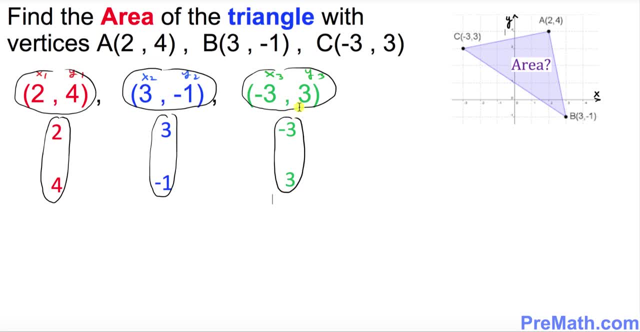 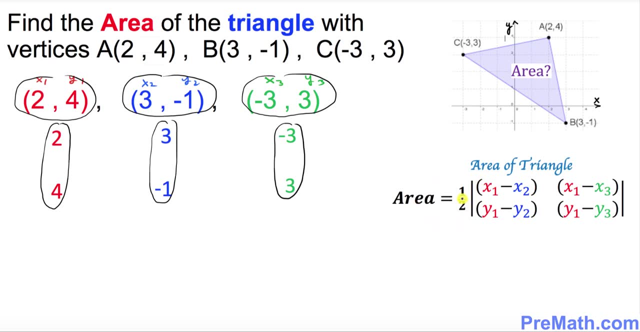 and y3. And this is a vertical position. And here's the area of the triangle formula that we will be using. And if, even if- you don't want to use this formula, I'll show you another easy way that even you don't need this formula. So see how I'm gonna do that one. And finally, now we're. 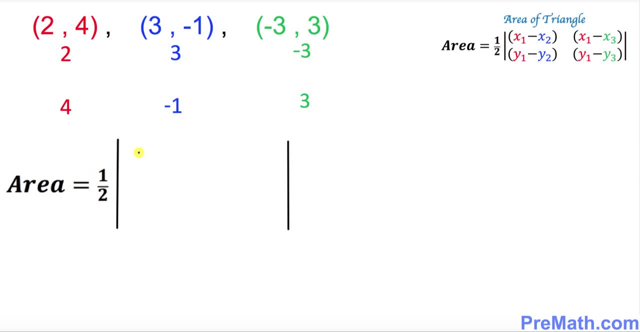 gonna be finding the area of the triangle by just filling out this box And, by the way this: you see these two vertical lines. this box is closely related to a matrix And we call this one a determinant. So this box is called determinant, So let's go ahead and fill out the 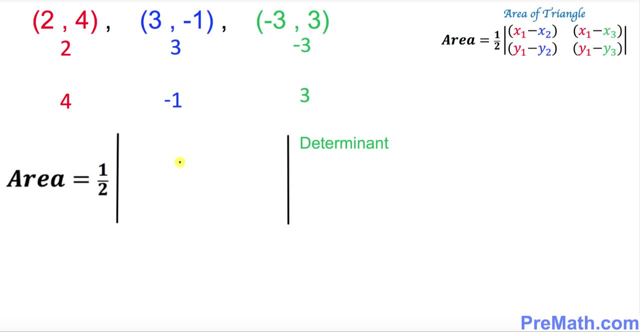 values over here, the entries in this box, And here I have filled out these numbers. As you can see, these red numbers showed up in two columns over here and over here as well, and this blue right up here just once, and this green just once on the right hand side. so the next step is: i want 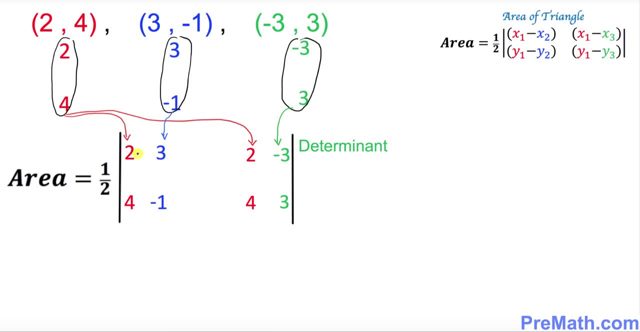 you to just put: look at these numbers two and three. i want you to put a minus sign in between, always minus sign in between these numbers, minus sign and minus sign. so far, so good. let's go ahead and simplify this thing. so this is equal to the area, equals to a half times. let's go ahead and